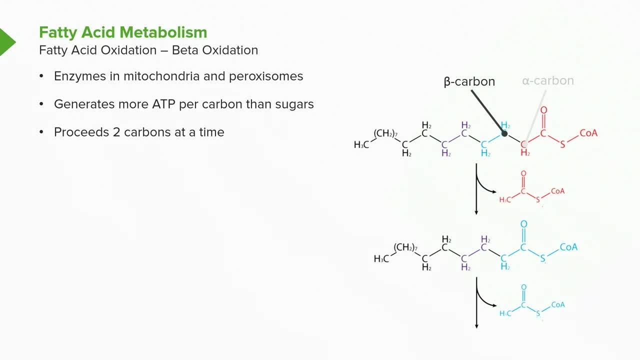 carbons, numbers two and three, so either term is commonly used. That breakdown process, as I said, releases a single acetyl-CoA, that's a two-carbon piece, and then continues along at two carbons at a time. Now, fatty acid oxidation is a multi-step process, like most metabolic pathways, but 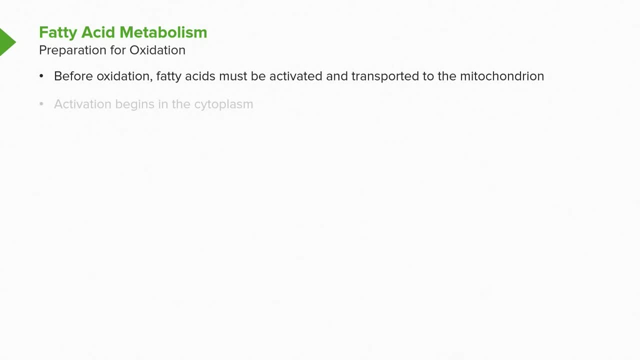 there has to be some processing of the fatty acids to get them ready for the oxidation. Fatty acids that start in the cytoplasm have to first be activated and then moved into the mitochondrion. but as we will see, that process is a little odd. The activation of 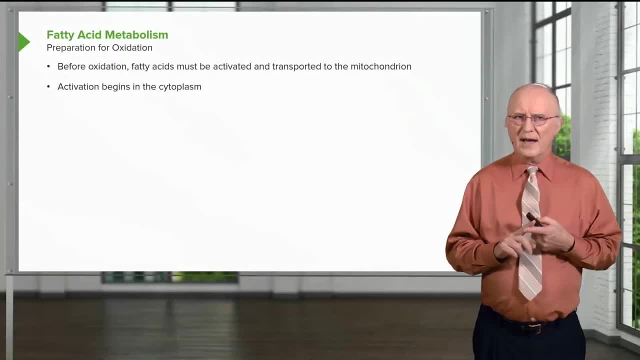 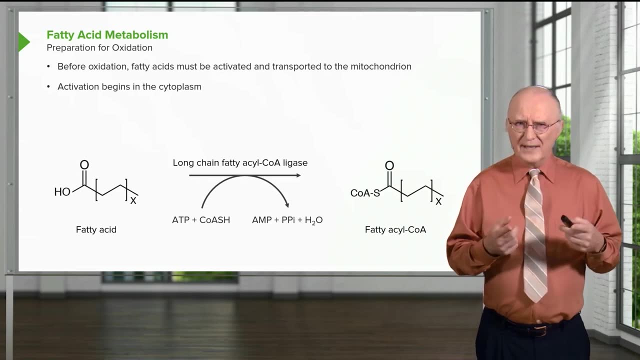 a fatty acid begins in the cytoplasm and this involves the attachment of a fatty acid to the cytoplasm, So the fatty acid is a molecule called coenzyme A or, as people more commonly say, CoA. This is an energy-requiring step and you can see that ATP energy is needed to do this, and 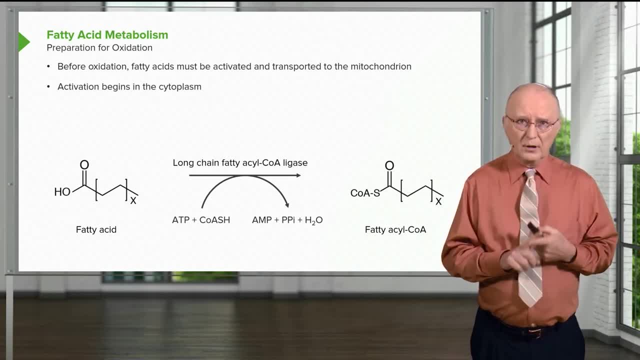 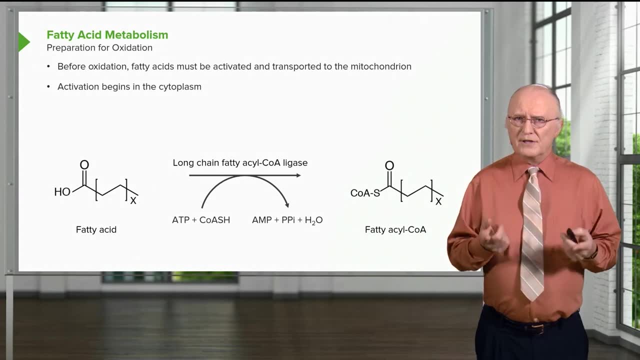 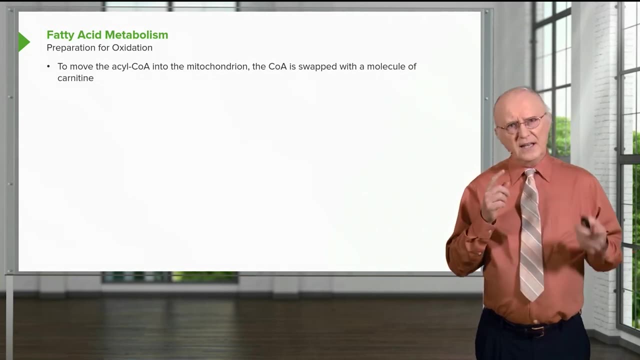 the product of this is not ADP, as we've seen many times before, but actually AMP, and that's a reflection of the fact that this is a pretty high-energy bond that's being created. The result of this action is a molecule called fatty acyl-CoA. Now fatty acyl-CoA needs to get. 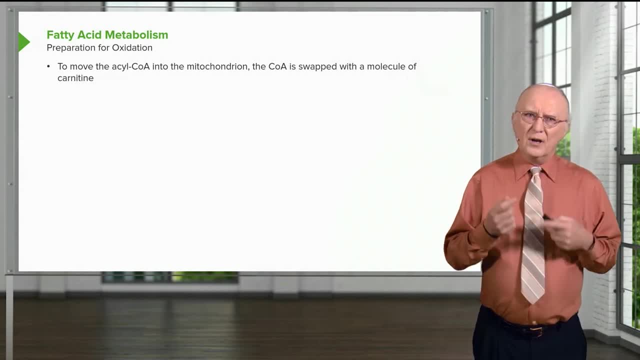 into the mitochondrion where the oxidation occurs. but there's a little complication with that: The acyl-CoA won't directly go into the mitochondrion. so the cell has wasted some energy in some thought by putting this CoA onto the acyl-CoA, and then we see it. 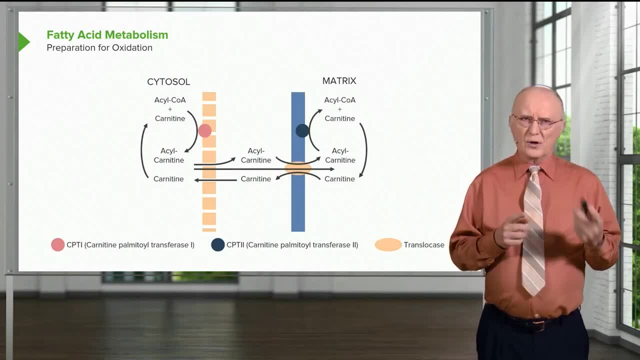 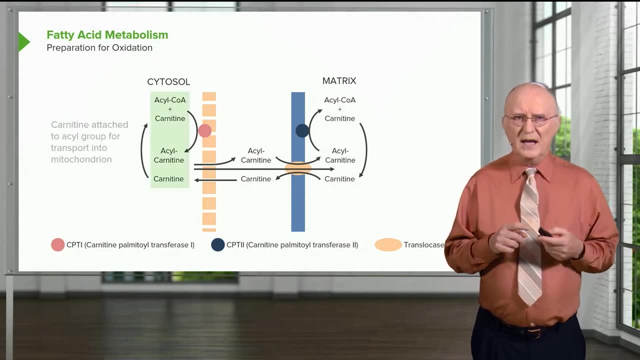 gets taken off. So in the next step of the process, starting in the cytoplasm on the left, we see that the acyl-CoA is combined with a molecule called carnitine to make an acyl-carnitine. Now 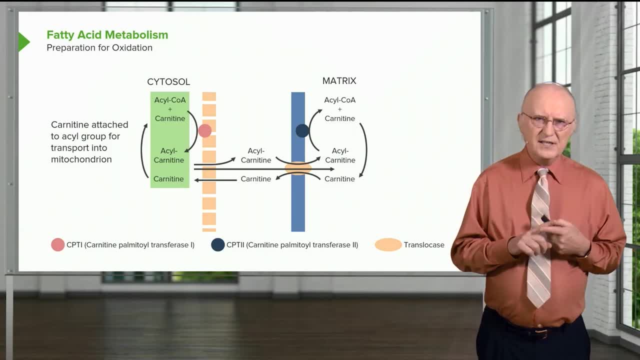 this step is essential for the movement of the acyl group into the mitochondrion and the reason is: is the CoA just can't make that move across the lipid bilayer? I should also mention that we're looking at the mitochondrion here, So on the right side, where it says: 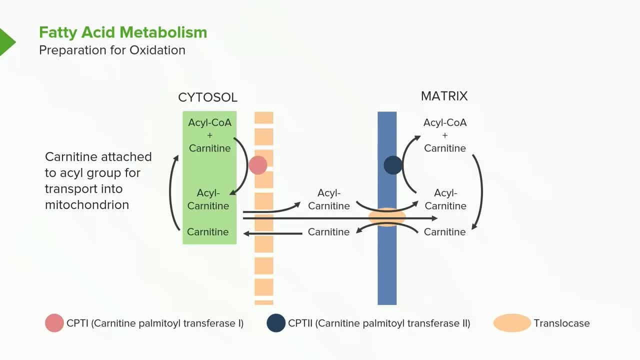 matrix, we're talking about the inside of the mitochondrion and, of course, on the left side, where it says cytosol, we're talking about the cytoplasm of the cell. In between the two you see the yellow and blue lines that are drawn there and those. 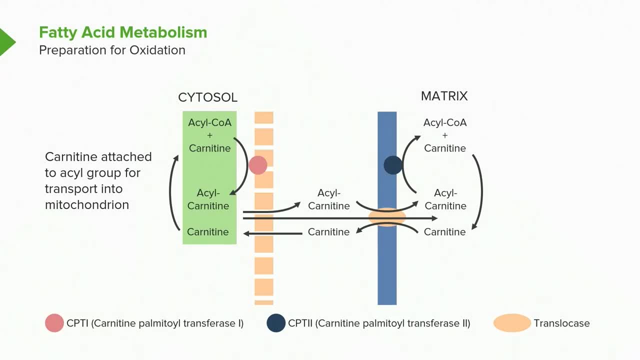 relate to two layers of membrane covering the mitochondrion, the yellow one being what's called the outer layer and the blue one. what's the inner layer? The blue one is very impermeable to a lot of substances, whereas the yellow one is fairly permeable. 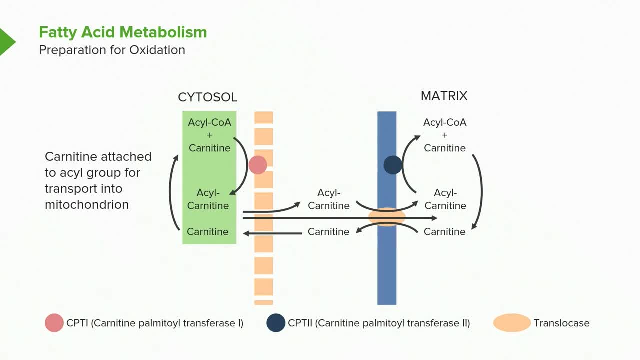 So you see the acyl-carnitine moving into what's called the intermembrane space, the space between the yellow and the blue lines, and then, when it gets there, it encounters the yellow protein. there, that is a transfer protein that physically moves the acyl-carnitine. 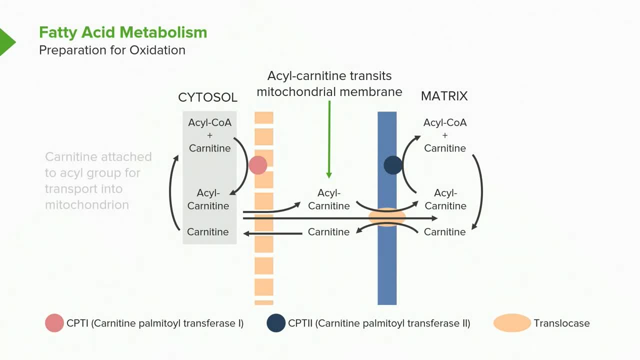 into the mitochondrial matrix. as you see Now, once it gets in the mitochondrion, then the reverse of all this process actually happens. The CoA that was floating around the mitochondrion is now attached to the acyl group and the 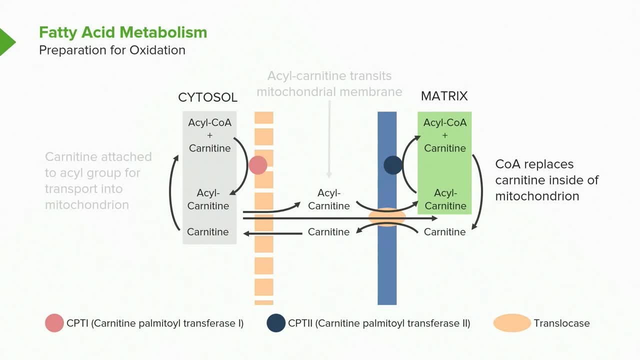 carnitine is released. The carnitine ultimately makes it back out into the cytoplasm and the process continues. So what we've done here is what we describe as a shuttle. The shuttle has carried the acyl group from the cytoplasm into the mitochondrion. We have an acyl-CoA in there and the acyl-CoA. 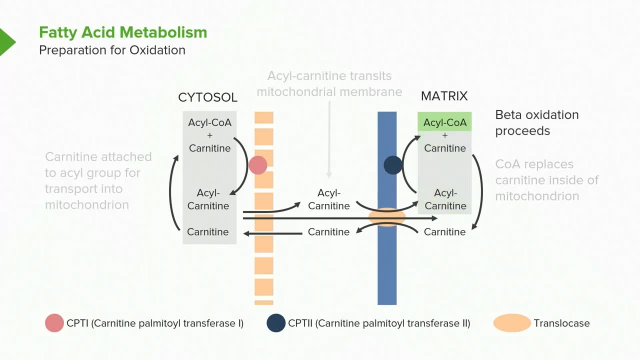 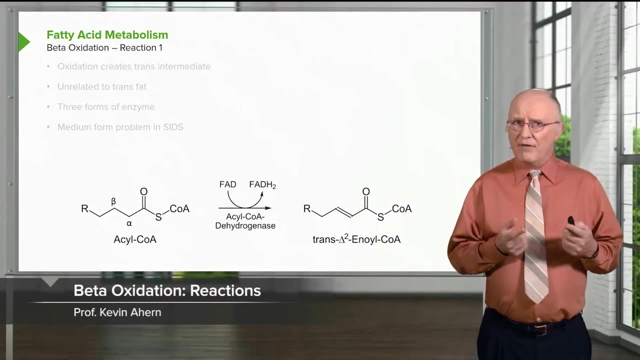 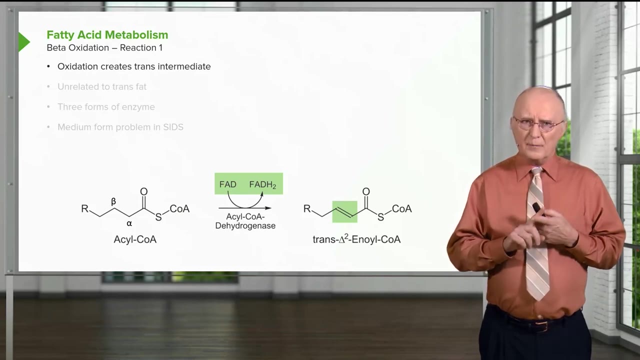 is the target for the oxidation. Beta-oxidation proceeds now, starting with that acyl-CoA. So we see now the step-by-step process whereby a fatty acid is oxidized. The oxidation in this process is shown in the first step. below We see an enzyme called acyl-CoA dehydrogenase. 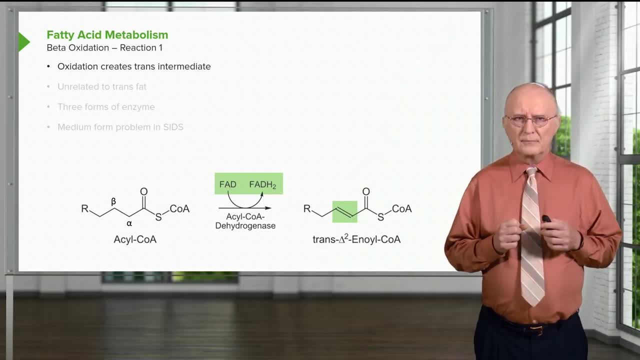 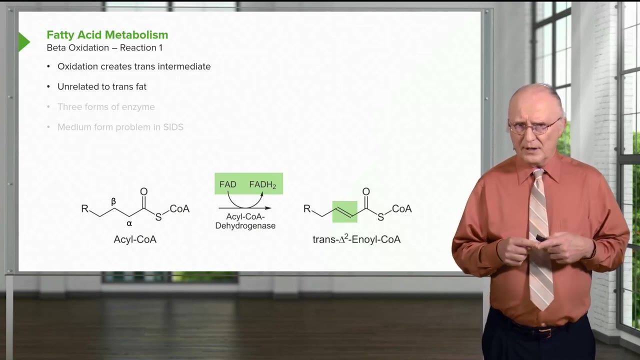 and it does the very first reaction on that fatty acid. You can see that all the action in fatty acid oxidation occurs between carbons, two and three, Or the alpha and beta, depending upon how you call it. The first oxidation is the removal of electrons and protons and those are donated to FAD to make FADH2.. The result of that oxidation 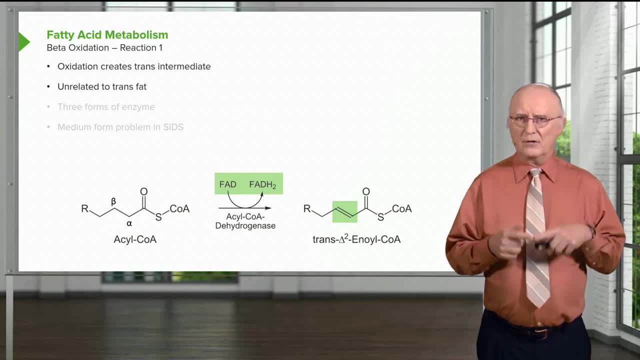 creates a trans-bonded fatty acid called trans-delta-2-enoyl-CoA. That name isn't very commonly used, by the way, But the important thing is it's a trans-fatty acid, And I note that it's not related to. 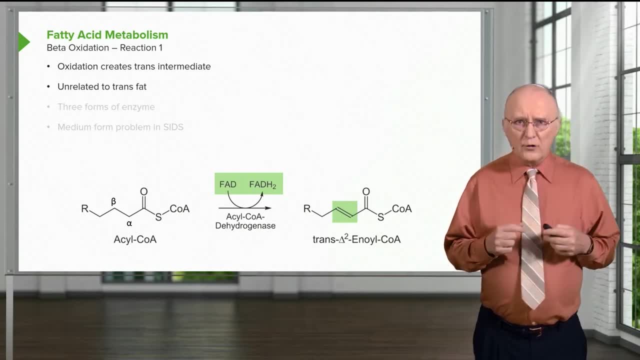 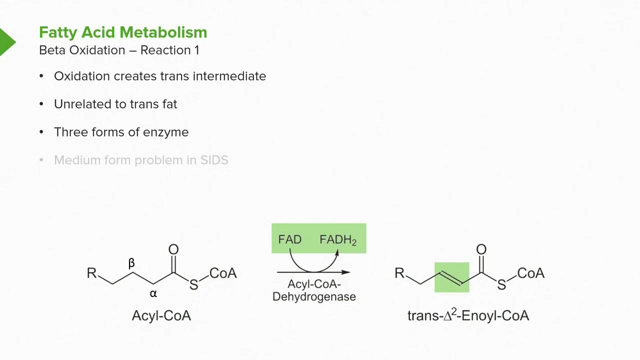 trans-fat. Trans-fat happens. Trans-fats are as made for other reasons. This is a normal intermediate in fatty acid degradation. Trans-fat is typically made by chemical treatment of food. Now, there are three forms of this enzyme. There's a form that works on long fatty acids. 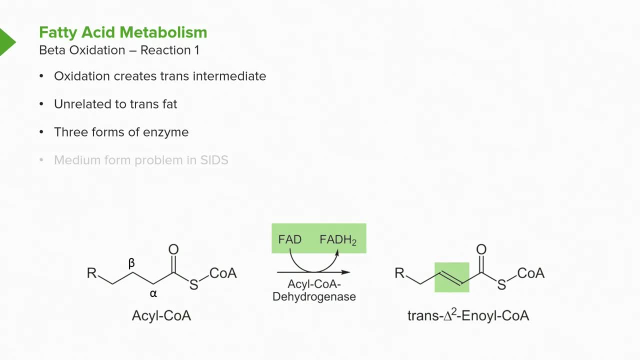 typically longer than about 20 or so, A form that works on medium-sized fatty acids, between about 18 and 10 carbons. And then there's a form that works on short fatty acids, typically less than 10 carbons. Now, of note, the acyl-CoA dehydrogenase that works on the medium form of the acid, is a 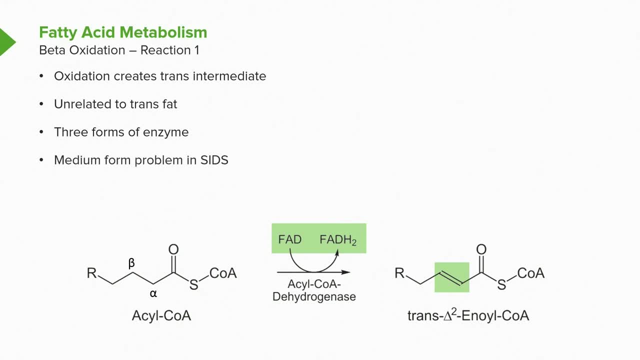 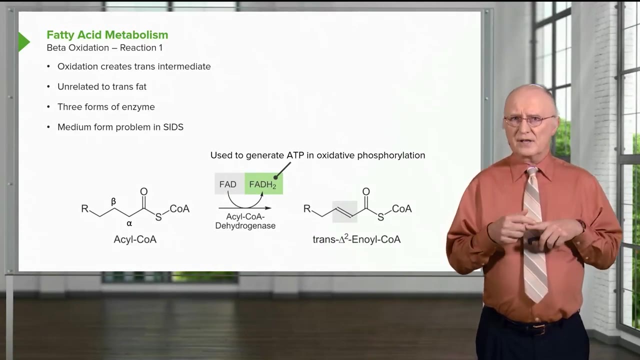 form that is absent in infants who have died from Sudden Infant Death Syndrome. Now it's not a cause-effect, but there appears to be a relationship between the absence of this enzyme and SIDS. Now the FADH2 that was generated in this process can be taken into oxidative phosphorylation. 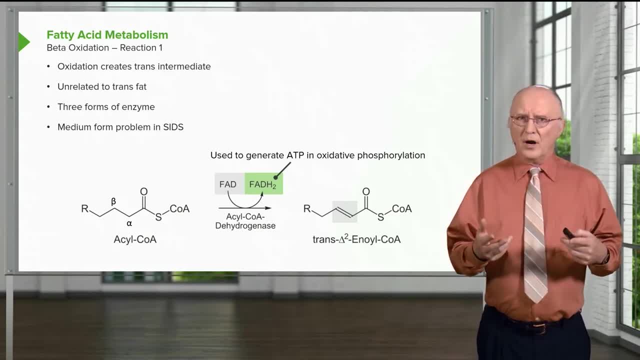 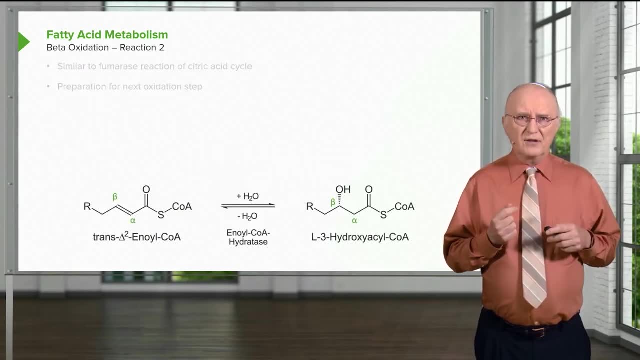 and used to make ATP. So we're seeing that these oxidative processes are used to generate energy that the cell can use for other purposes. Now, in the second reaction of fatty acid oxidation, we see that this trans-intermediate gets a water added across it. This is a very common reaction in organic chemistry and is catalyzed. 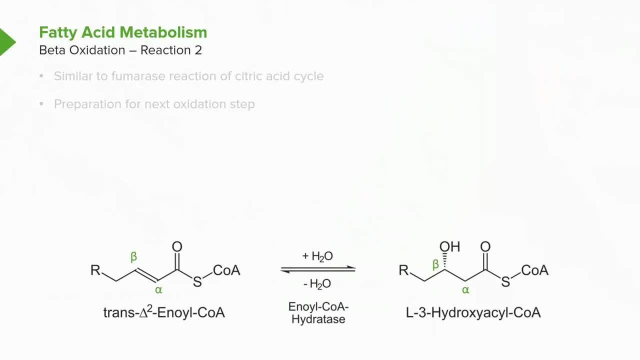 by the enzyme enoyl-CoA hydratase. This enoyl-CoA hydratase creates a molecule that has a hydroxyl group on the beta carbon or carbon number 3, and that hydroxyl group is in the L configuration. 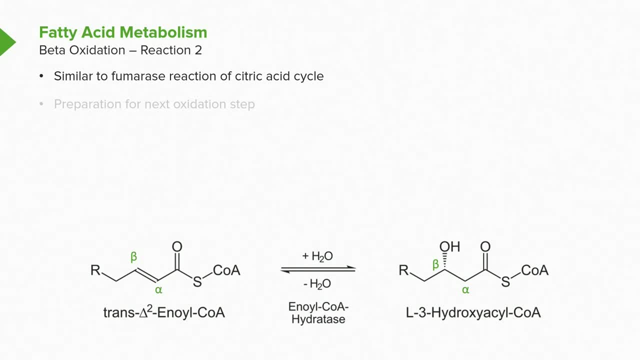 as you can see here Now, this reaction is similar to a reaction that occurs in the citric acid cycle. In fact, this reaction and the next two reactions are very similar to citric acid cycle reactions, And this allows for an oxidation that will occur in the next step. 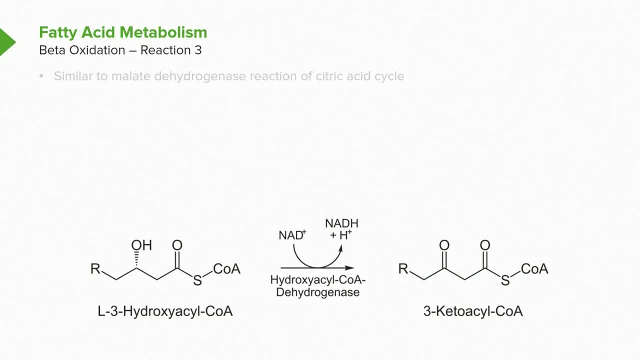 So the second oxidation of fatty acid, fatty acyl-CoAs, occurs by the process that you can see here On the bottom. you see that we have the hydroxyl fatty acid that we created on the last stage And on this step we see that that hydroxyl group is converted into a ketone. That oxidation, 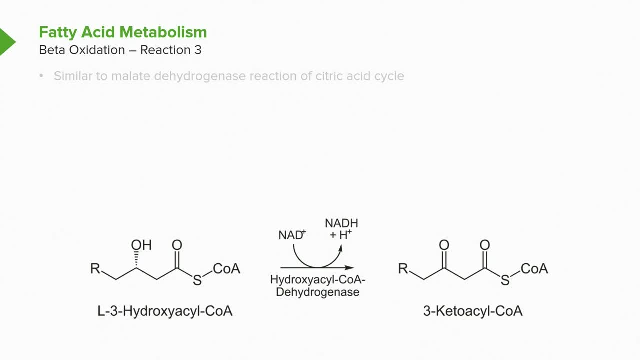 is catalyzed by the enzyme that you see on the screen and causes production of NADH plus H plus. that is the transfer of electrons and protons, as we have seen before. Now this reaction is similar to the malate dehydrogenase reaction of the citric acid. 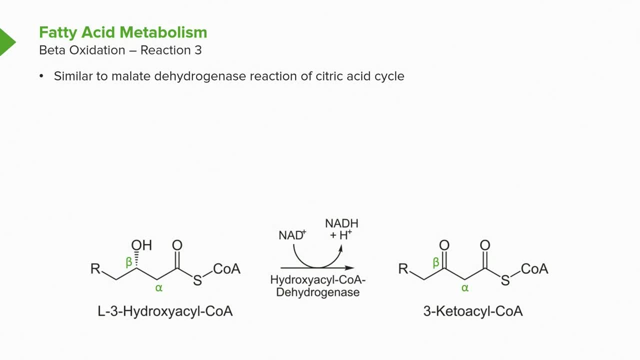 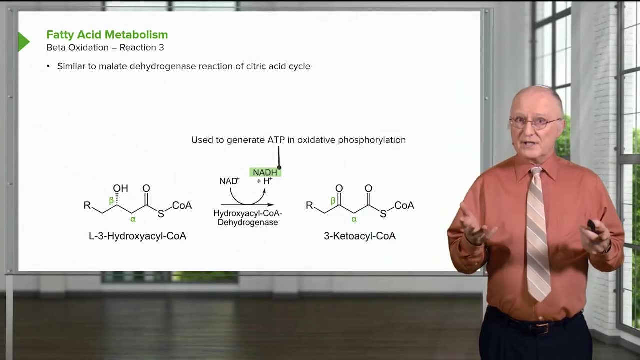 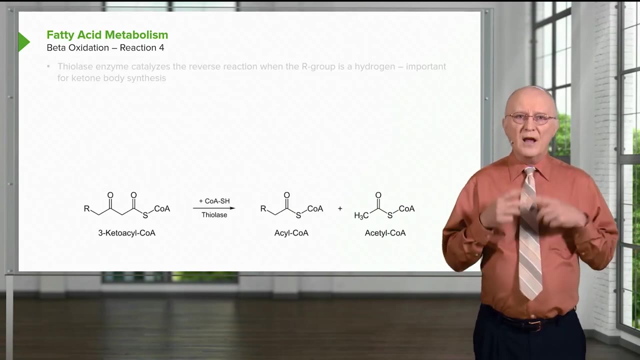 cycle. This reaction is preparing us for the final step, in which we are going to have to actually cleave the fatty acid into two pieces. The NADH, of course, like the FADH2, can be used to generate ATP and oxidative phosphorylation.